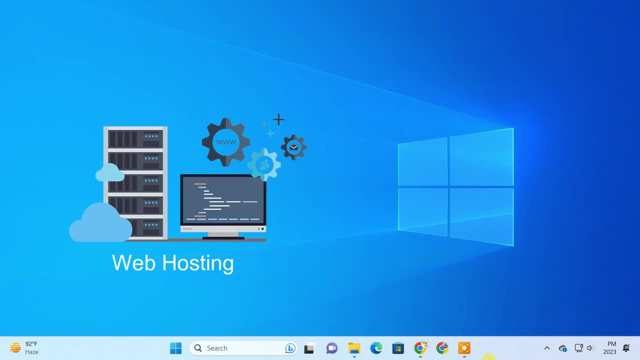 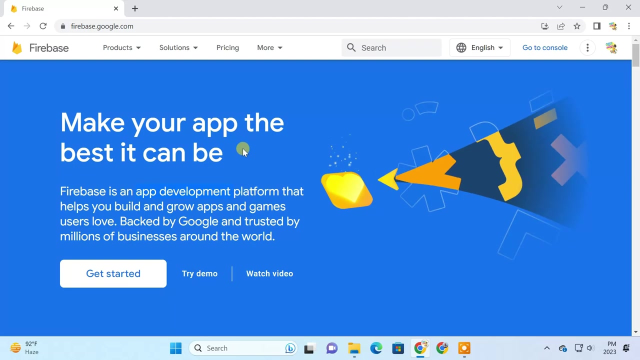 Web Hostings come with a monthly or yearly premium and are good for business purposes. But if you want to host a personal static website with a few daily visitors, then you don't need to purchase any web hosting. You can use Google Firebase, which provides hosting for free. Google Firebase is a mobile app development. 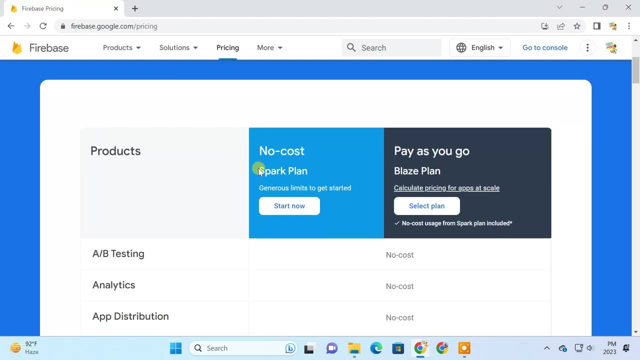 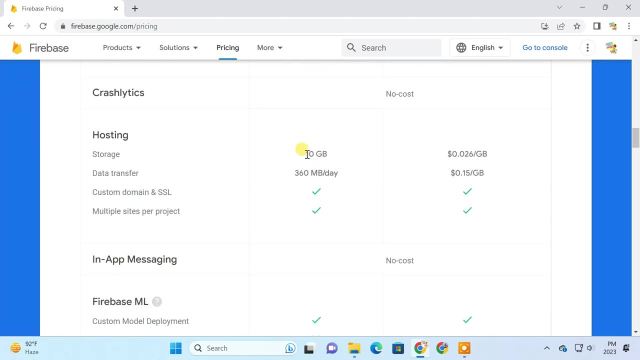 platform. It offers a Spark plan which includes free web hosting for lifetime at no cost. However, it has some limitations. You can only store 10GB of data And it has a data transfer limit of 360MB per day. It means if your webpage size is, let's say, 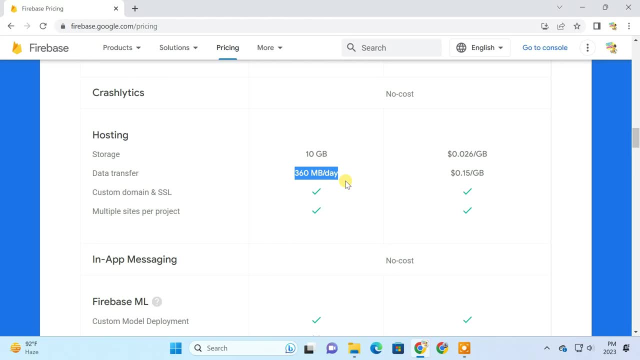 1MB, then it will allow 360 visits per day. This is enough for a personal website with little to no user base. This is also useful for beginner developers who want to present their projects for all to see. The best part is, you can add your custom domain. 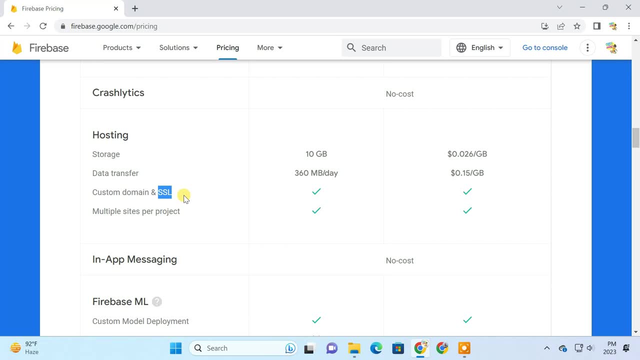 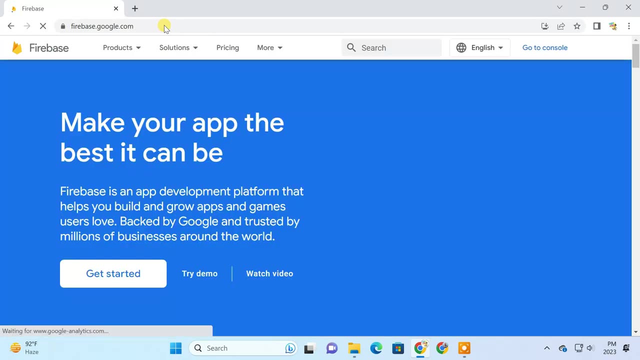 with a SSL certificate free of cost. So let's get started. Let's see how you can host a static website with a custom domain and SSL on Google Firebase. First of all visit firebasegooglecom, Then sign in with your email account. 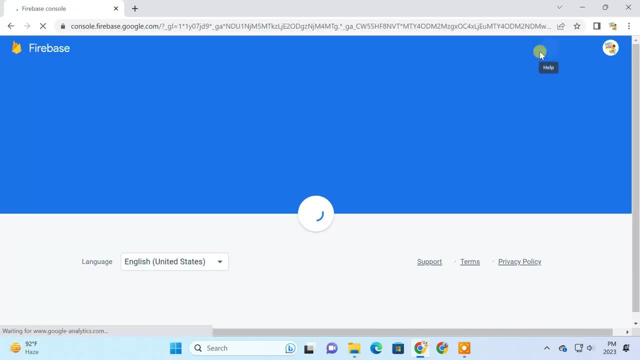 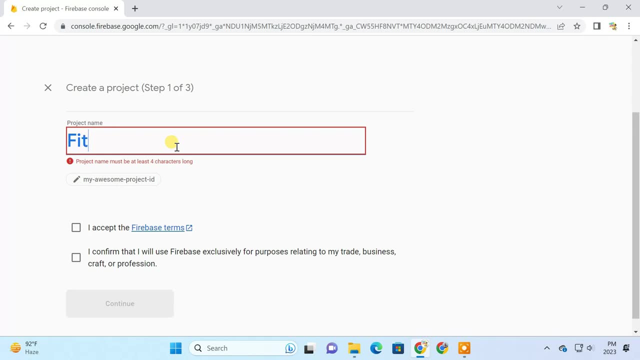 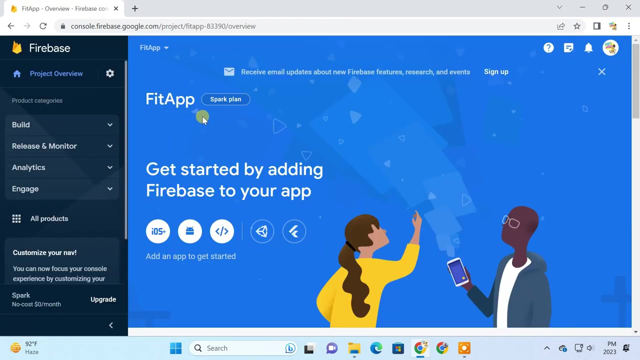 To create a new project, go to console. Click on create a project. Enter your project name. You can create an affix with firebase doc and name. Once the project is created, you are ready to host your website with firebase hosting. 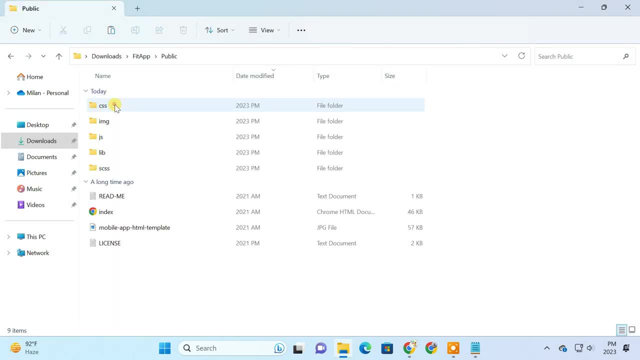 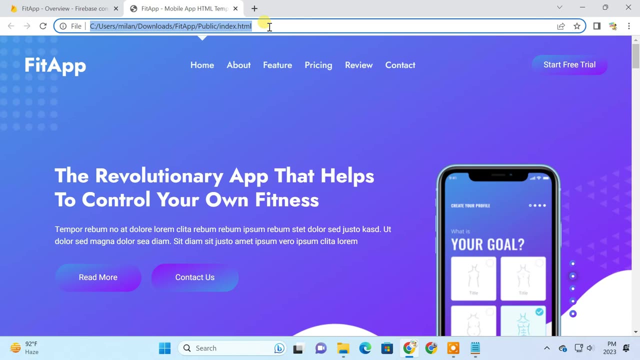 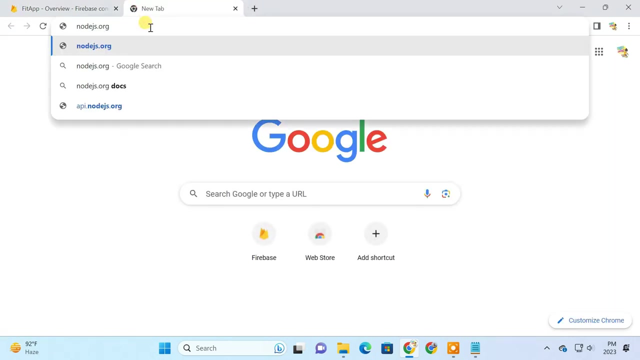 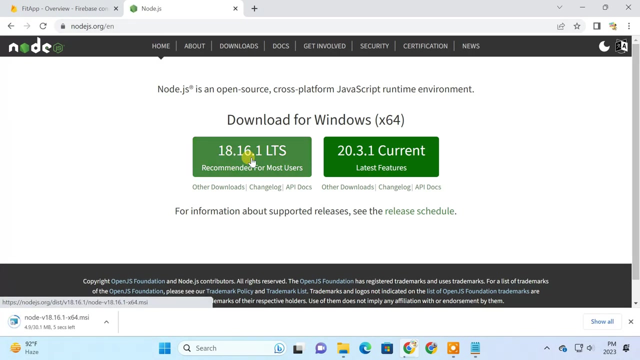 I already have a static website on my computer. To deploy this site on the firebase hosting, we need to use the felt ability firebase command line tool, also known as firebase cli. before you can install the firebase cli, you need to install nodejs on your computer. visit nodejsorg and download the nodejs installer. 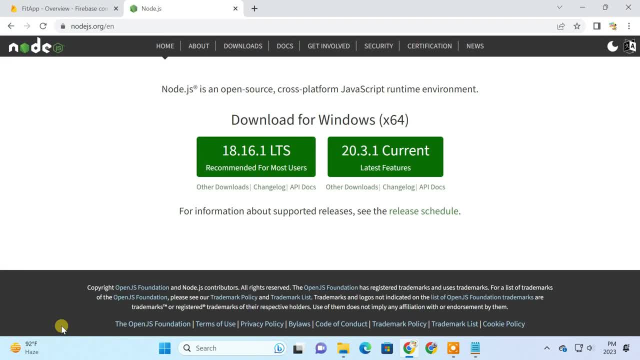 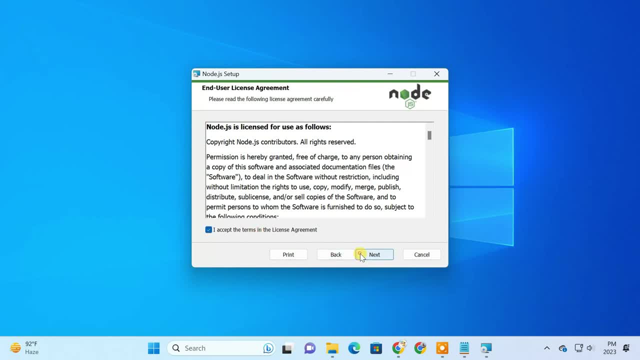 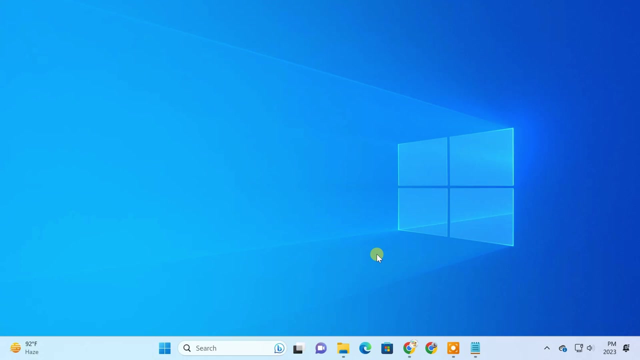 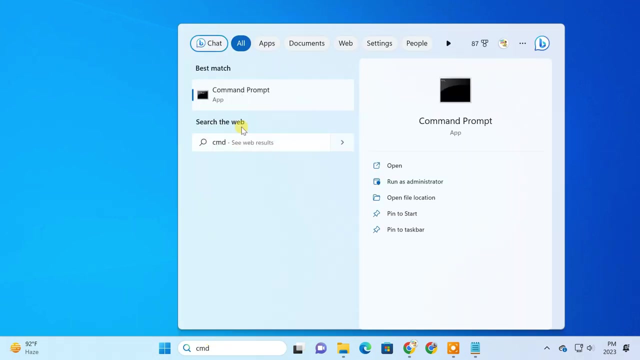 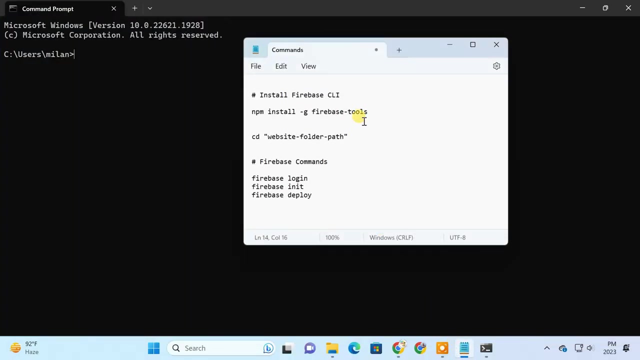 for your computer, then install it on your computer. once you have installed nordjs, you can now install firebase cli using the nordjs package manager. for that we just need to run a simple command to do so. open command prompt. run this command to install firebase cli on your device. 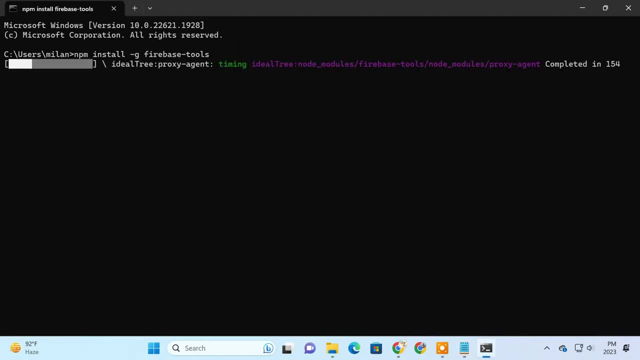 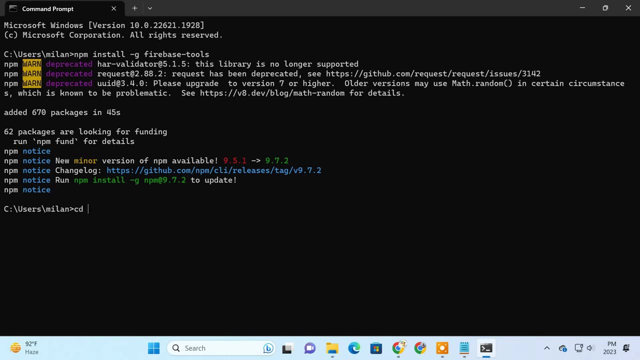 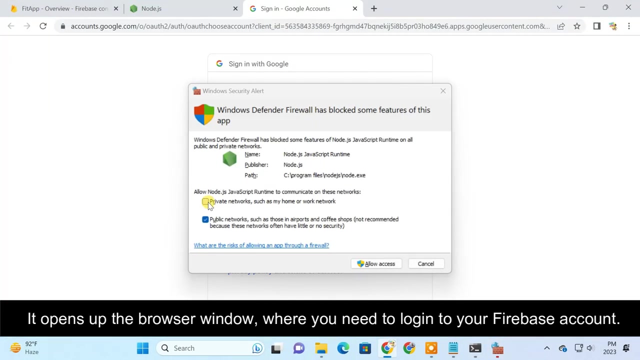 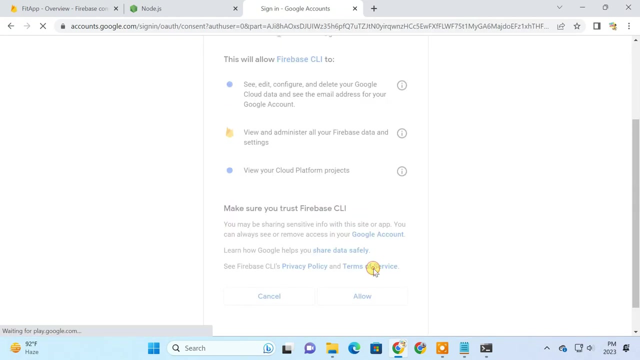 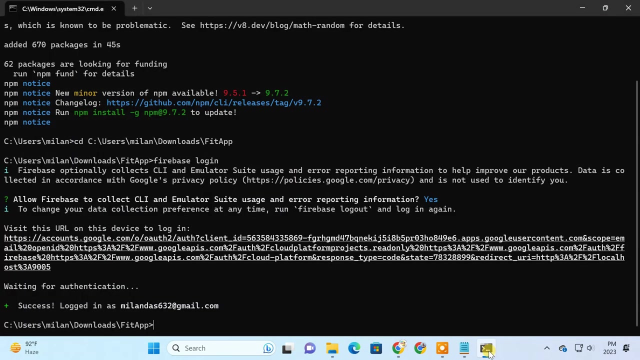 so, After successful installation, go to your project folder. After that, run this command to login to your firebase account. Once you have successfully logged in, it will show you this message in your browser. Now, to initiate a firebase project, you have to enter this command. 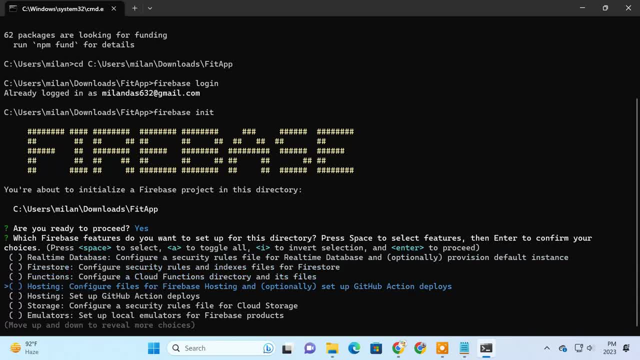 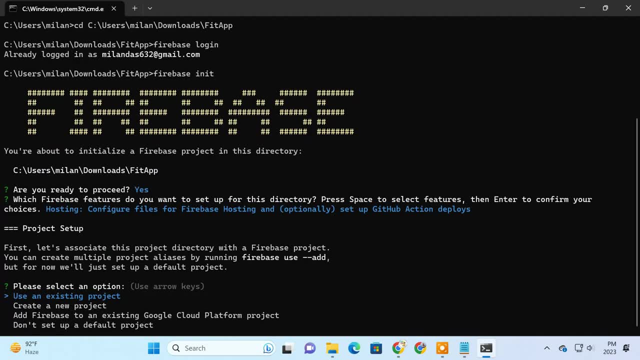 Here we have to select the hosting feature, since we are using it only for hosting purposes. Then press the spacebar to select it and press enter to go to the next step. Then it will ask you to select your project, Select your firebase project. 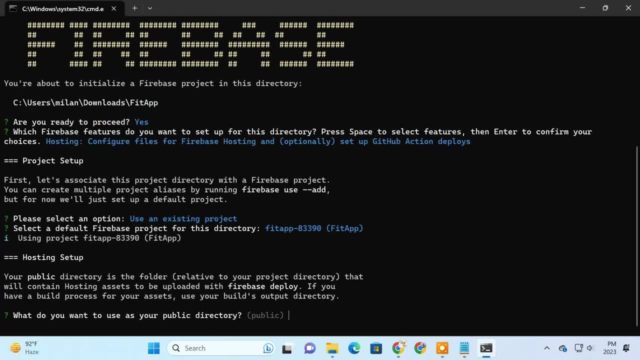 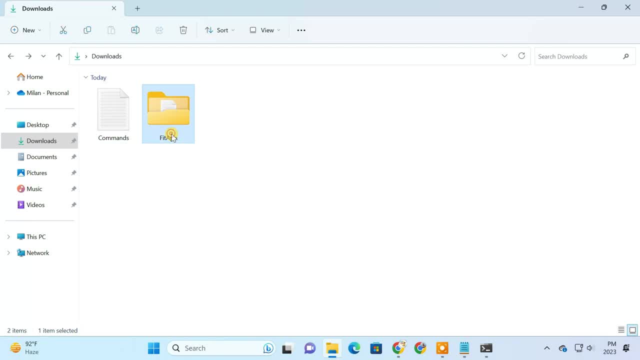 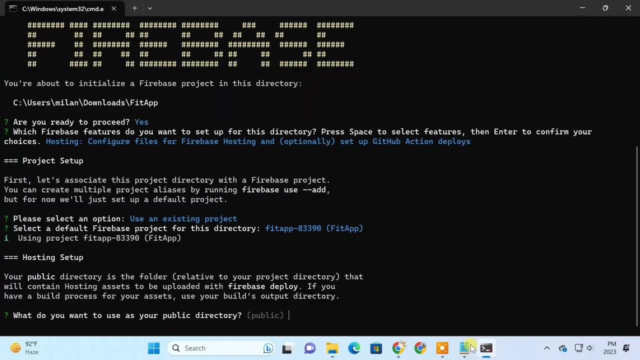 Select the project which you created earlier. Then it will ask you to enter the main folder in which all your website assets are present. In my case, it's the public folder. Now it asks whether the site is a single page or not. I'll enter y. 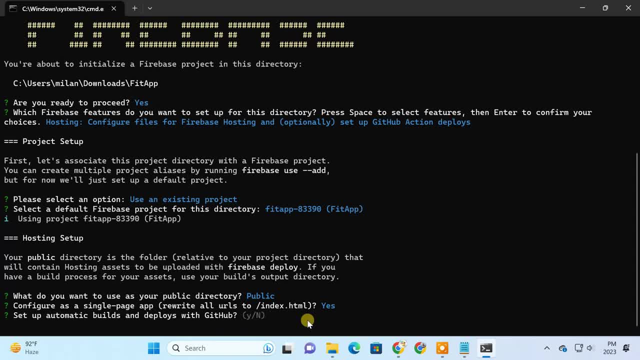 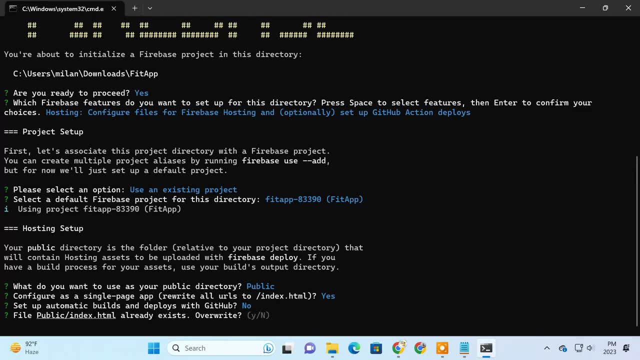 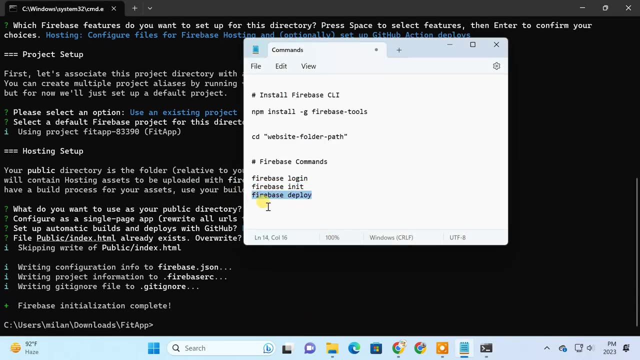 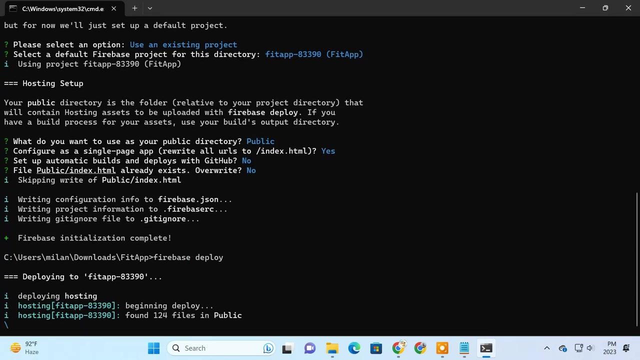 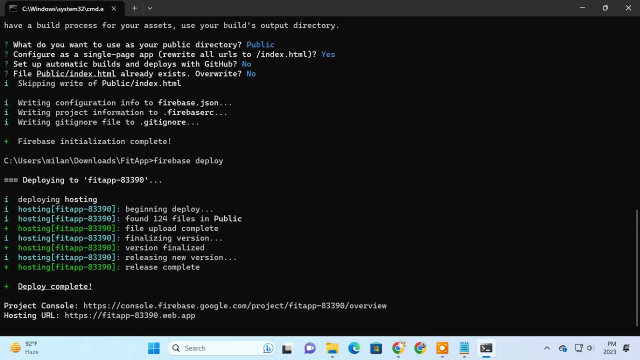 We don't need to use the GitHub development, so enter n. It will try to override your indexhtml file. To avoid doing that, enter n. Finally, for the deployment of your project, you have to run this command. Now your website should be live. 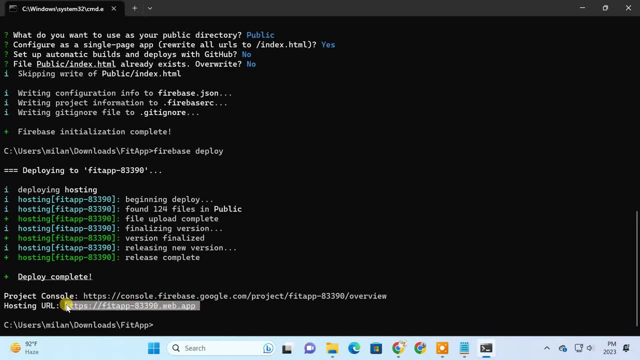 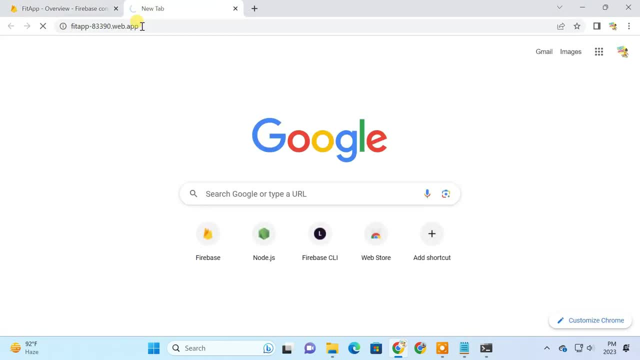 It provides the website URL here. You can check by opening this URL in your browser. Now, it's running. It's running. You can check by opening this URL in your browser. It's running. Although it's not going to run on this site, I've saved it. 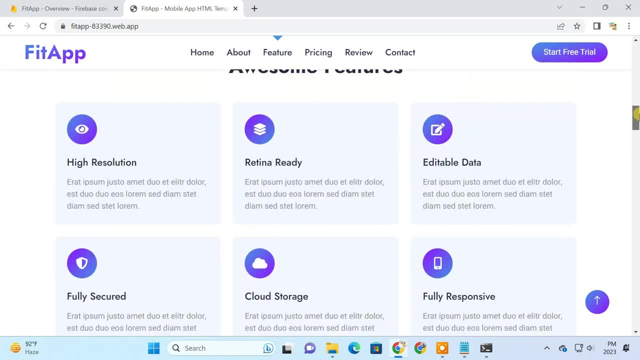 I'll ask it to run on the site. It'll seeds that this site is running in. It'll see that it's running on the site. You can check this and then it'll say: in this case it's running And in this case it's running in the same location. I'll change the admin to admin. It'll say mls to be on the site where I'm running. Let's get the archHave said. I'll check it and see if it's running on the site. In my case it's running on the site. 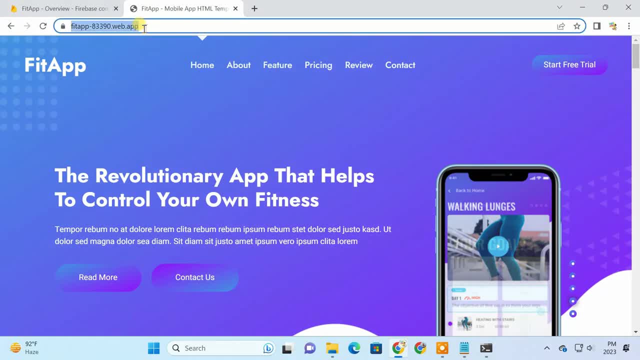 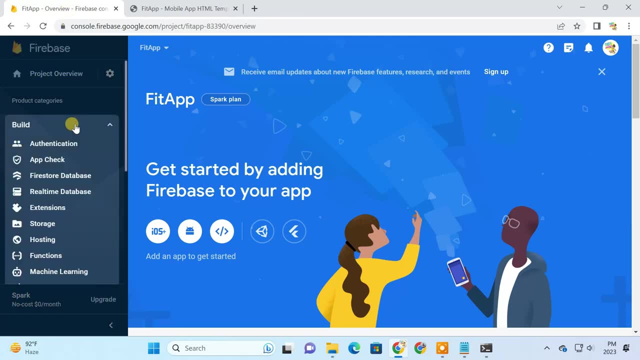 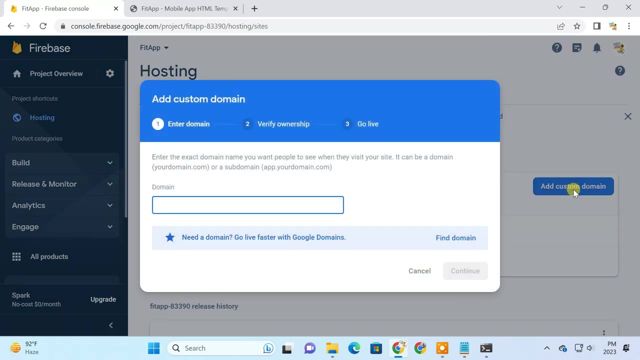 Once your website is public, you can replace this domain with your custom domain. To do that, go to your project in the firebase console On the side menu. click the build tab, Then click on hosting. Click on add custom domain, Then enter your domain name. 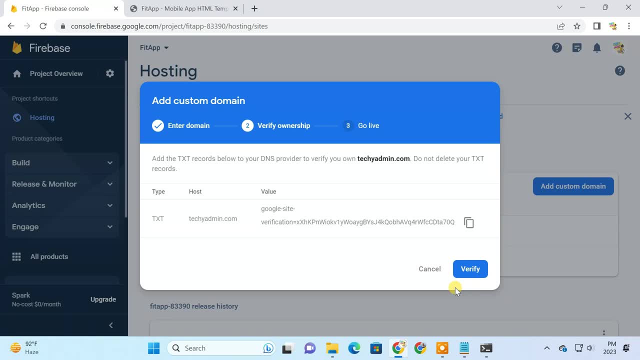 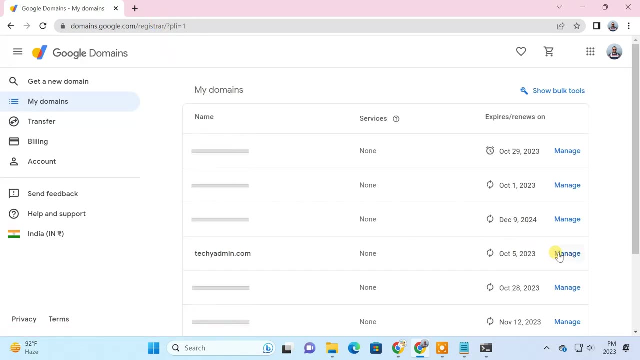 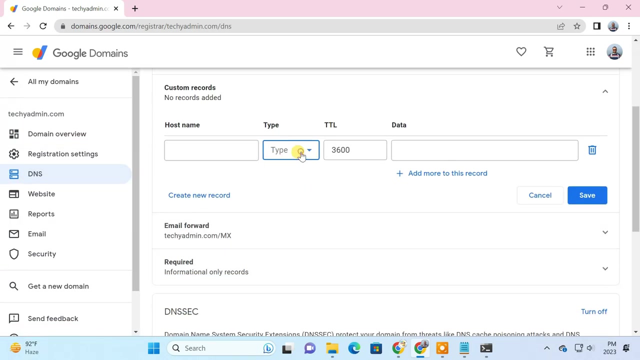 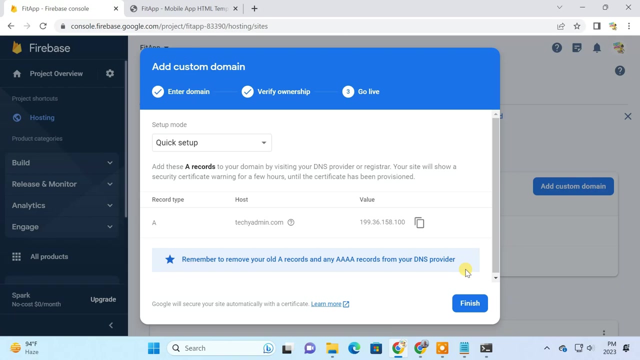 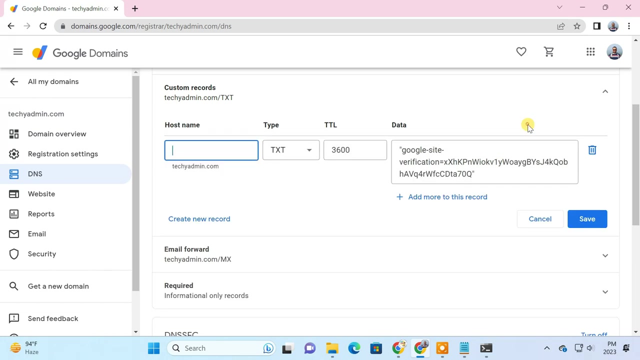 First you need to verify your domain ownership. To do that, add this txt record to your domain provider's dns. I purchased this domain from google domains. Let's quickly update the txt record there. So here it is. Next, to connect the domain to firebase hosting, you need to add this a-record to your domain's.